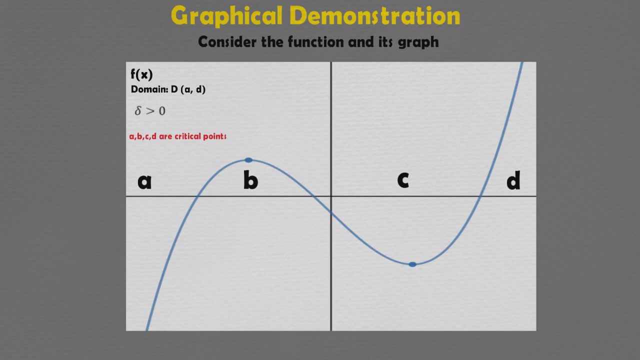 derivative of function either does not exist or is zero. Critical points are the location at which local minimum, local maximum, absolute minimum and absolute maximum values occur. Therefore, in the present example, we will look for values at these locations by applying different conditions. Consider an interval about critical point a: The interval. 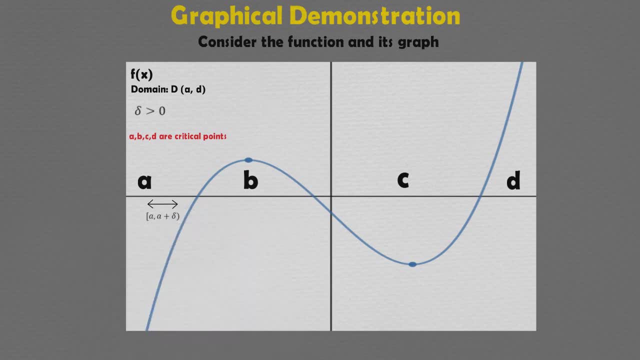 is from a to a plus delta. So it is a small interval, including critical point a. Similarly, consider an interval about critical point b. The interval is from b minus delta to b plus delta. Here the interval is from a to a plus delta. Here the interval is from a to a plus delta. 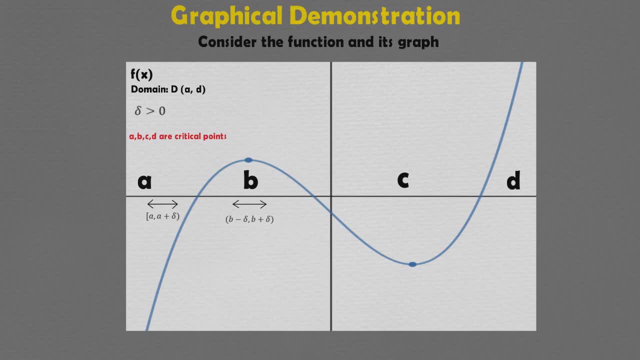 Normal is an open interval which can also be taken as a close interval. So it does not matter whether you take it as a close interval or an open interval. So it is the second interval, including critical point p. Similarly, consider an interval about a critical point c, The 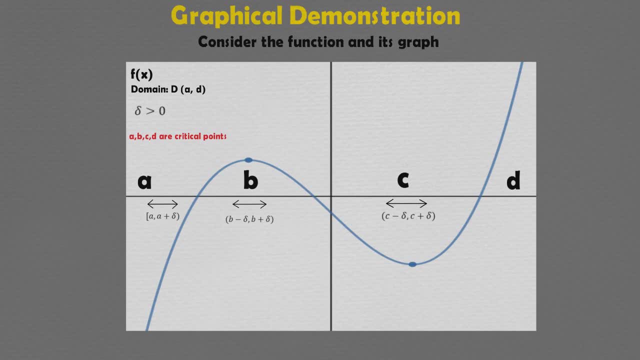 interval is from c minus delta to c plus delta, So it is the third interval including critical point c. Consider another interval about a critical point d. The interval is from repay: То這個是 tchê 4 för су clHi k for� delta. 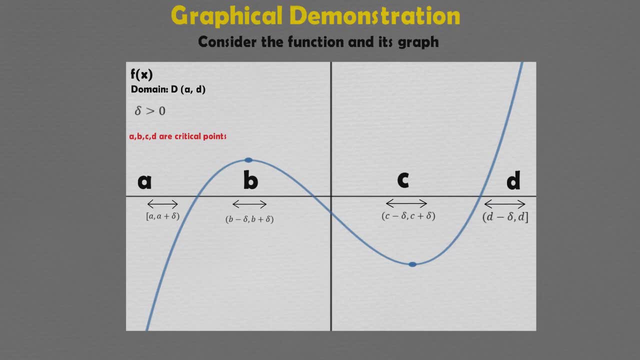 minus Delta to KCöz's delta Liberalism. So it is the fourth interval, including critical point D. Let's analyze interval 1, that is, from a to a. plus delta At this interval. if you look at the graph, at a the willow function is the lowest, which. 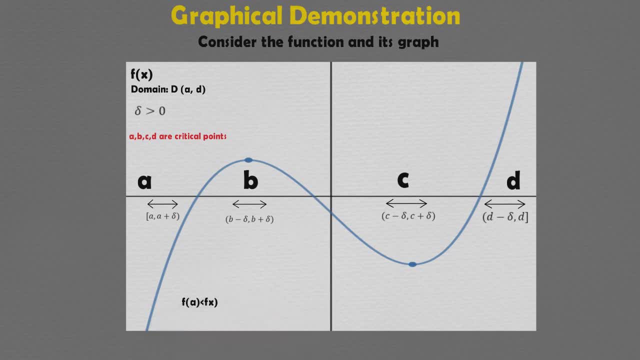 is f of a. That is, f of a is less than f of x in this interval. So by definition it is the local minimum point and f of a is the local minimum value. Similarly, analyzing interval 2, that is, from b minus delta to b plus delta, 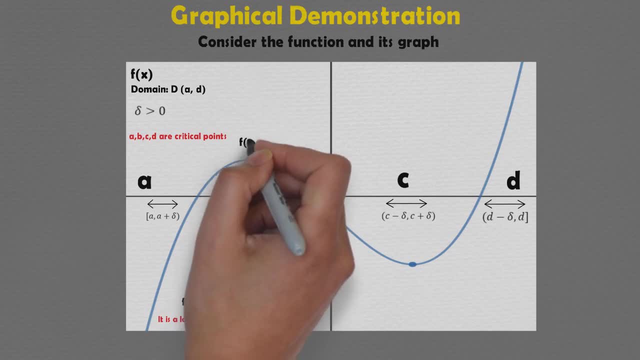 In this interval. at b the willow function is the maximum which is f of b, That is, f of v is greater than f of x in this interval. So by definition it is the local maximum point. Similarly for interval 3, that is, from c minus delta to c plus delta. 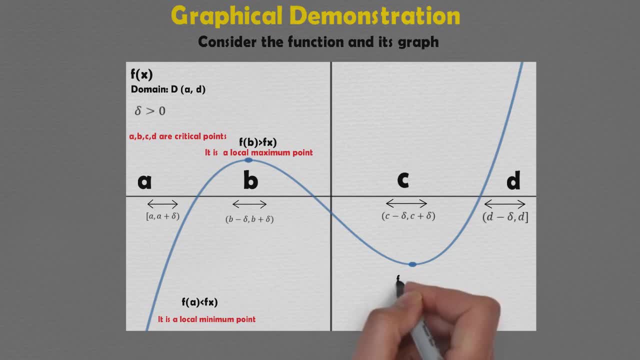 At c the willow function is the lowest in the interval, That is, f of c is less than f of x in this interval. So by definition it is the local minimum And f of c is the local minimum value For interval 4,, that is, from d minus delta to d. 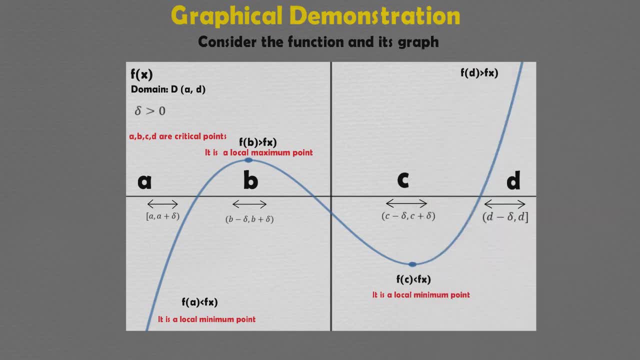 At d the willow function is the maximum, That is, f of d is greater than f of x in this whole interval. So by definition it is the local maximum point and f of d is the local maximum value. So that's how you identify local minimum and local maximum value of function from the graph. 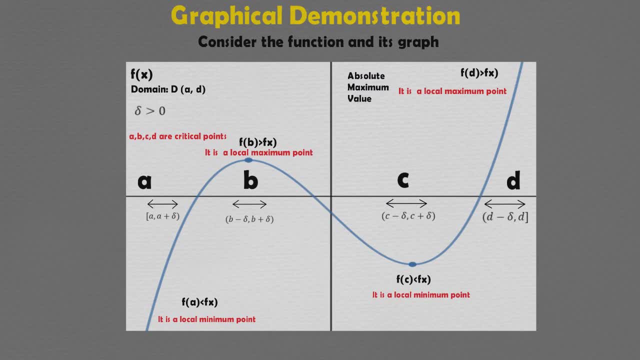 Now absolute maximum, which is the greatest willow function in the entire domain. Here the domain is from a to d And by looking at the graph, absolute maximum occurs at d and its value is f of d, Because f of d is the maximum value of the function in the entire domain. 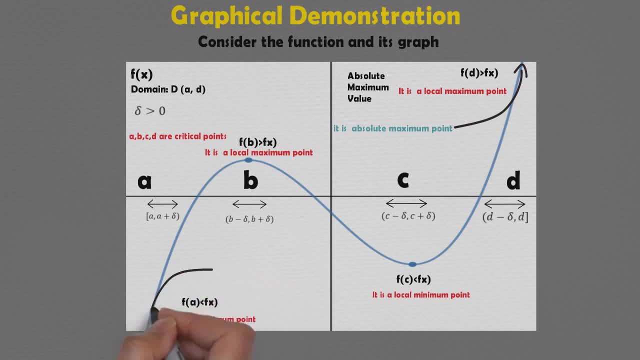 Therefore it is absolute maximum value. Similarly, absolute minimum is the lowest value in the entire domain, which in this case occurs at a and its value is f of a. So at point a both local minimum and absolute minimum occurs, And at point d both local maximum and absolute maximum occurs. 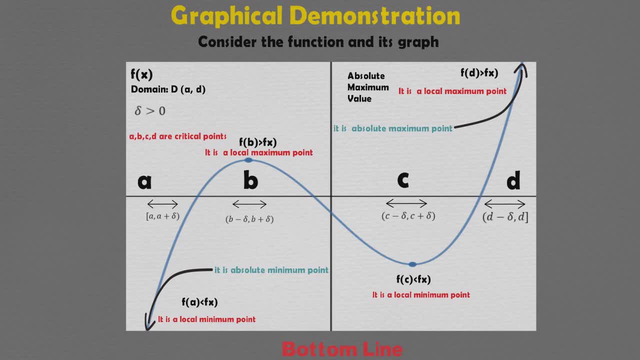 So the bottom line is: absolute maximum is also local maximum, but not every local maximum is absolute maximum, which is clear from the graph, because at d, the absolute maximum is also local maximum, but at b, the local maximum is not absolute maximum because we have only one. 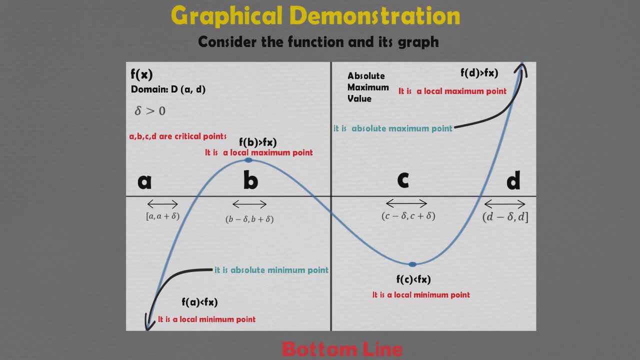 absolute maximum, and that is a- d. same is true for local minimum and absolute minimum values. that is, every absolute minimum is also local minimum, but every local minimum is not an absolute minimum. that is, at a, we have the absolute minimum, which is also local minimum, but at c we have the local. 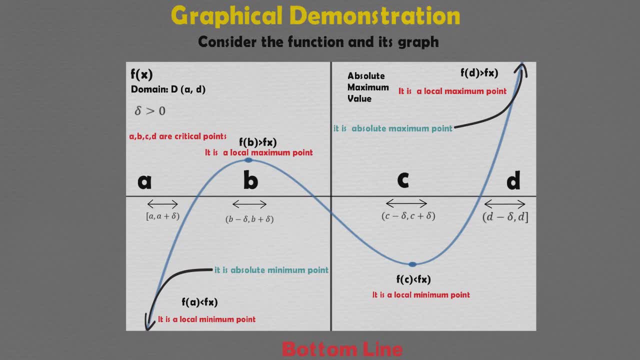 minimum, but it is not absolute minimum, because absolute minimum occurs at a and its value is f of a. there can be only one absolute minimum and one absolute maximum, but there can be multiple local minimum and local maximum values. what if we change the domain of the function from a to d? 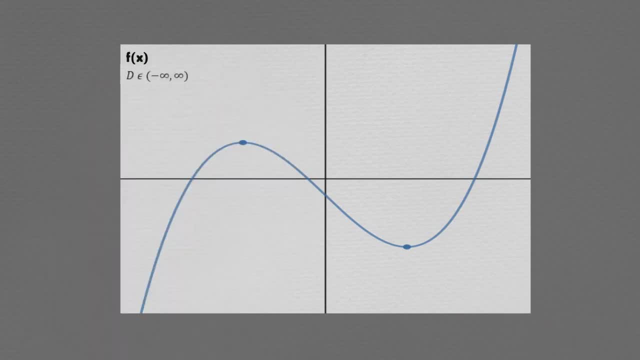 interval to minus infinity to infinity. in this case the critical points are b and c. only previously a and d were also critical points because derivative was undefined there as they were the endpoints of the interval, as the derivative did not exist at a and d. therefore they were the critical points and was analyzed for local and absolute minimum. and